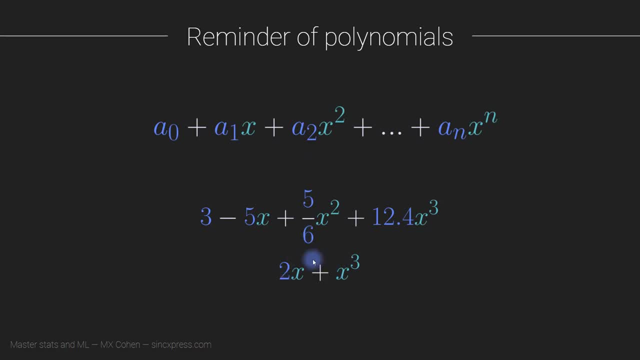 you know, think of writing 0 times x squared, but in practice that's just left out. Same thing with with a0, here is also set to 0.. So there's another concept in polynomials which is called the order. So the order of a polynomial is basically n. here It's the highest coefficient, So this is an nth. 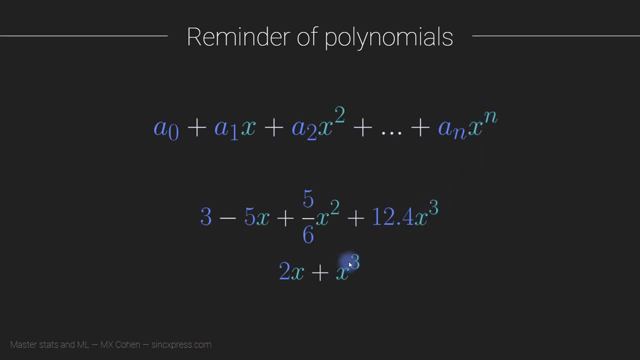 polynomial. This is a third order polynomial. This is also a third order polynomial. Sometimes people get confused about this because there's only two terms, But the order of a polynomial doesn't refer to the total number of terms. it refers to the largest exponent in any of the 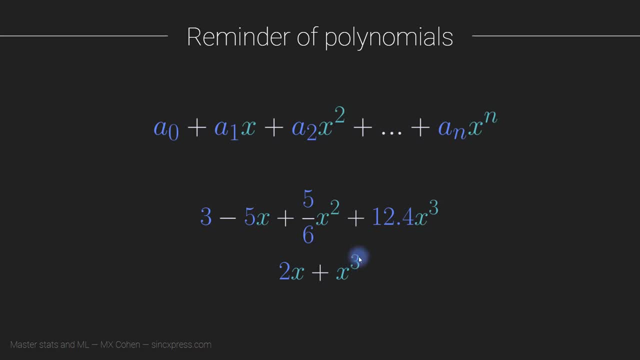 terms. So third order polynomial. Okay, so here's a polynomial regression. technically, This looks like the simple regression that you saw several videos ago, So you can see that the order of a polynomial is 0. So we can just say that this is a third order polynomial. We can also use this. exercise to write a polynomial. that's a polynomial, So the order of a polynomial would be: Vikings are- forgive me roughly, these are common austerity生活, H bars where an crispy littleättig. but maybe you take and then take some of that in and make them your isolating them so you offer. 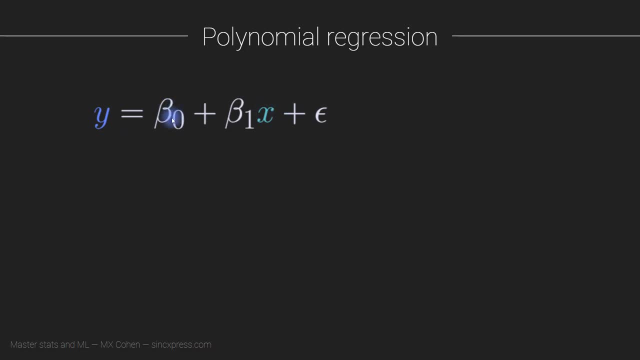 so here is a really common Toya, one polynomial you would create in closed class. You can allalu videos ago, But so you can see. this is beta zero times x to the zero which earlier I was calling a zero, now I call it beta zero, And now it's beta one times x to the power of one. So this simple. 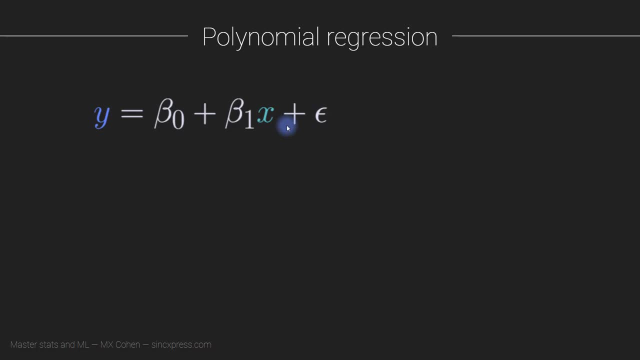 regression is actually nothing more than a first order. polynomial regression Okay, but with polynomial regressions we can add more terms here. So we can have something like this: So we say: y equals beta zero, the intercept plus beta one times x plus beta two times x squared plus. 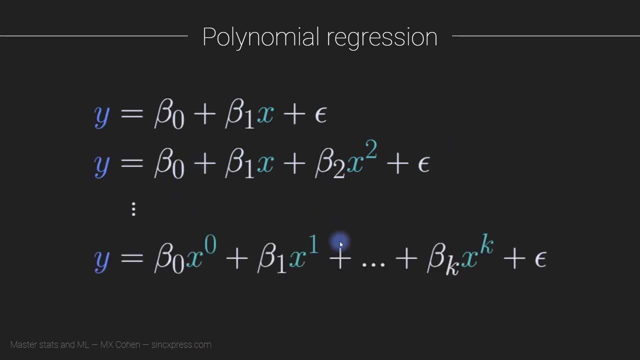 the residual term, and on and on and on, And so we can get this to be higher in order. So let's say beta k times x to the power of k, So this would be a kth order polynomial regression. Now here's a question: how can we fit this kind of model? look at these nonlinearities. 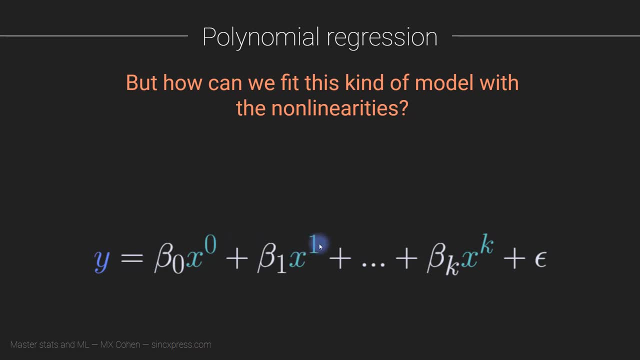 there's nonlinear terms, So you know these are here. x is linear, But now we're bringing x to higher and higher powers. And didn't I say in the beginning of this section that regression is all about a general linear model? So it has to be. 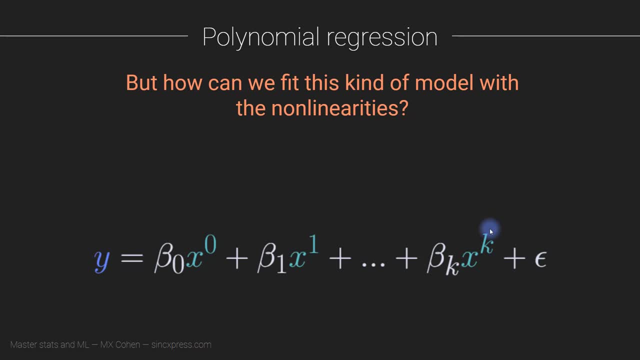 linear. So how can we fit this polynomial regression if we have these squared terms in here, which are in higher order, power terms which are nonlinear? Well, you have to remember the other thing I said about what needs to be linear and what can be nonlinear. So, in fact, the 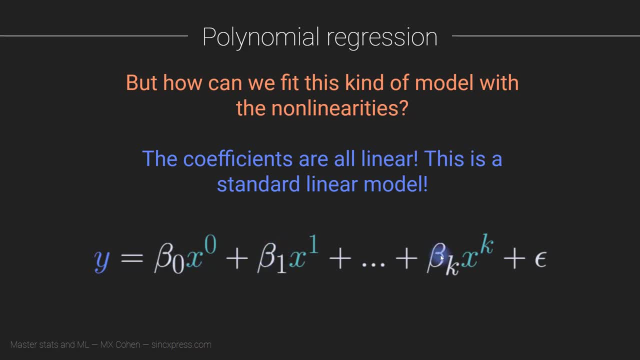 coefficient of the nonlinear regression is the coefficient of the nonlinear regression. So the coefficients are all linear. the betas are all linear. they're just being regular multiplied. there's no squaring happening to the beta. So in fact it may not look like it initially. 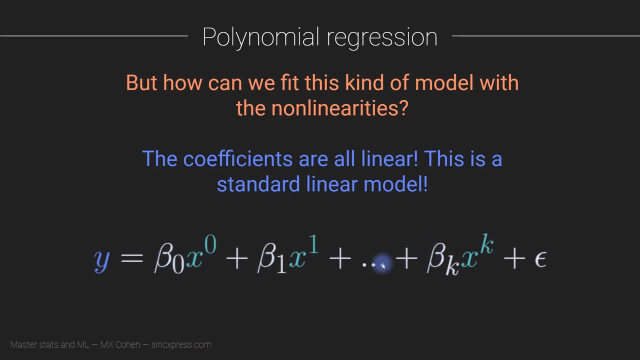 but a polynomial regression is a standard, regular run of the mill, vanilla, plain, general linear model. And that's because we're not doing anything nonlinear with the coefficients. It's just the data themselves that are getting raised to higher powers And that's why we're not doing anything nonlinear with the coefficients. It's just the data themselves that are getting raised to higher powers. 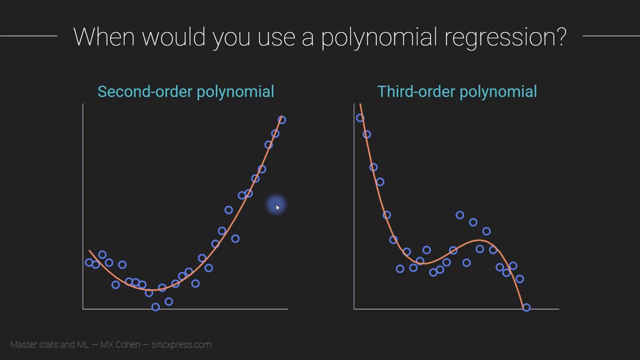 Okay, so here is what. here you see two examples. this shows you when you would use a polynomial regression. So here we have. our data looks like this: the blue circles are the data. blue circles are the data. So you can see that a line is not going to be a really great fit to this data set. 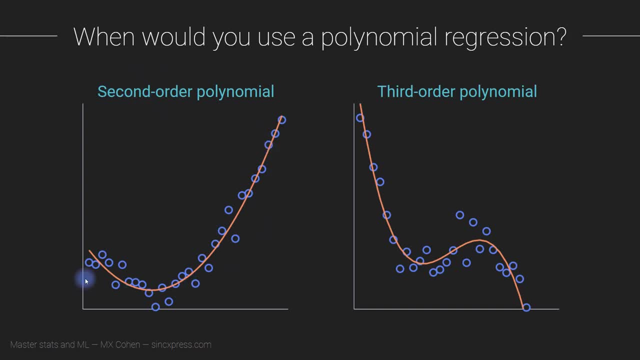 So this is a second order polynomial. So that means that this polynomial has the form y equals at beta one, which is the intercept, plus beta two times x, which is a linear term, plus beta three. Wait, I'm miscounting my betas. 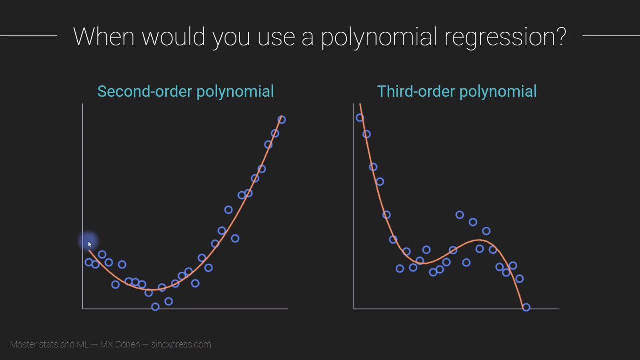 Anyway, beta two would be times x squared And that gives us this quadratic form here. So this part we need the x squared in here, the beta coefficient and the x squared in order to get this model to fit. And this will be a third order polynomial, So you'll probably recognize the. 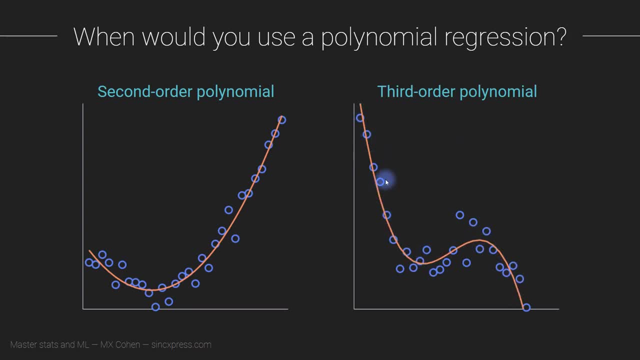 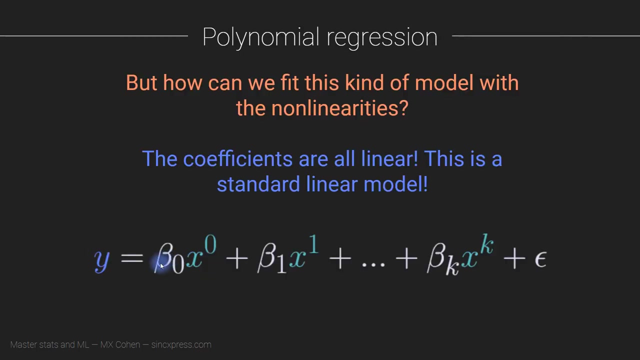 general form of x, cubed This dataset here. So these would be the kind of data that you would use for a polynomial regression. Now, of course, that leads to the natural question of what is the appropriate order, because when you, when you set up a polynomial regression, you are given: so this x, this is. 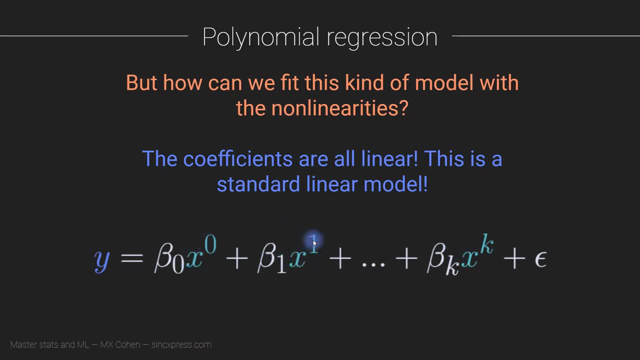 one independent variable. I can multiply, can bring it up to any higher power that I want. we could go up to, you know, beta 1000 times x to the power of two, So that would be equal to x squared, and so if I'm just going to take the value of two and I'm going to put this into the power of two. so I'm going to take this into the power of one and I'm going to take the value of two, And then you know. 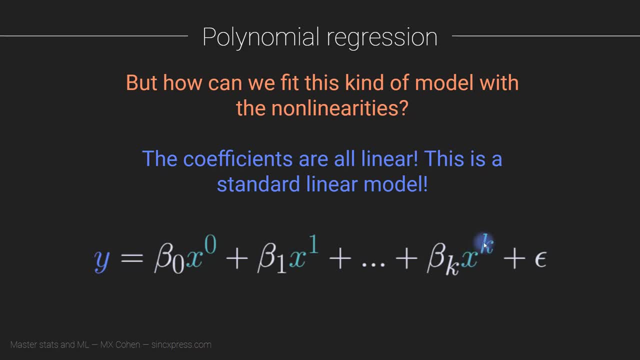 I can go up to just the values of x squared. So I can move it up and I can give it to something like this: 1,000 times x to the power of 1,000.. I mean, maybe that's a little high to be sensible. 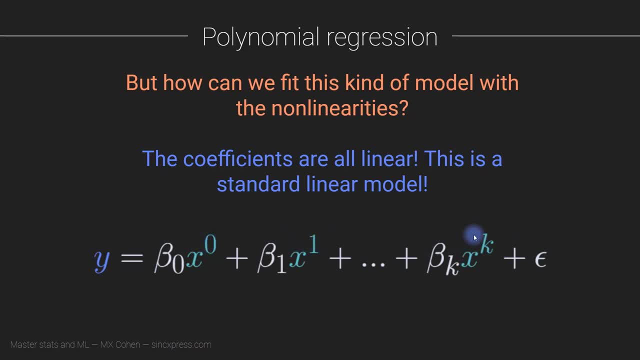 but you know there isn't a real hard limit for how many powers we can include here. I suppose you could say that the limit would be when k exceeds the number of data points, because then we can no longer fit the model. But that's only. it turns out to be just a soft constraint. 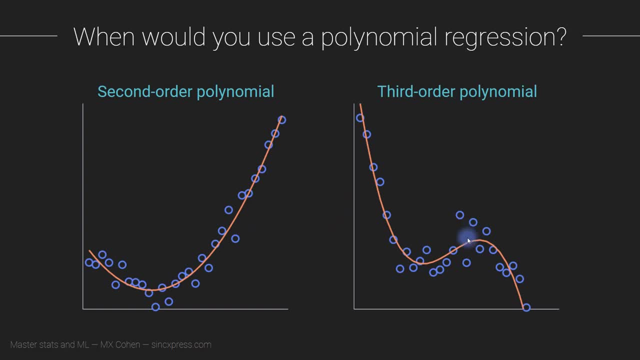 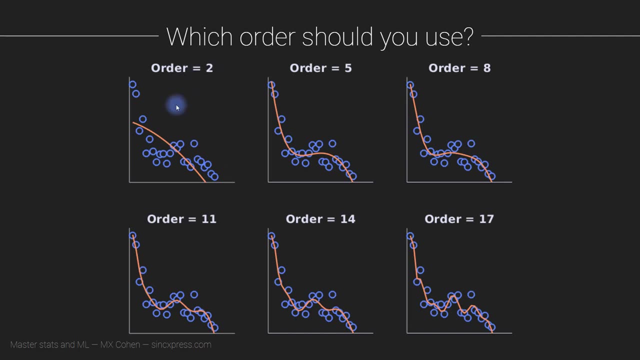 So how do we know what order the polynomial should be? So that's a good question. Here you see an example of this data set that I showed in the previous slide with an order of two. So visually this doesn't look good, right? 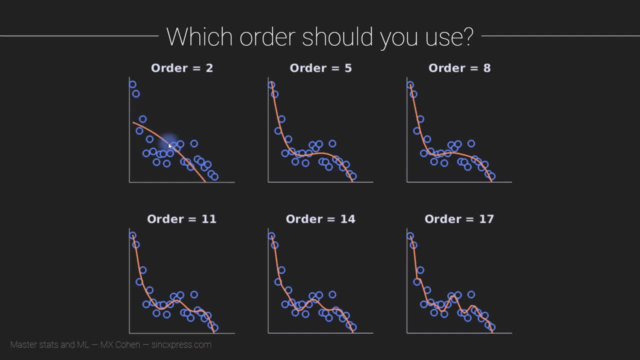 I mean we can. it's trying. you know the model is trying to fit the data. It gets an A for effort, but you know this is just not a good model And here we have increasingly higher orders. So here we have a model order of 17.. 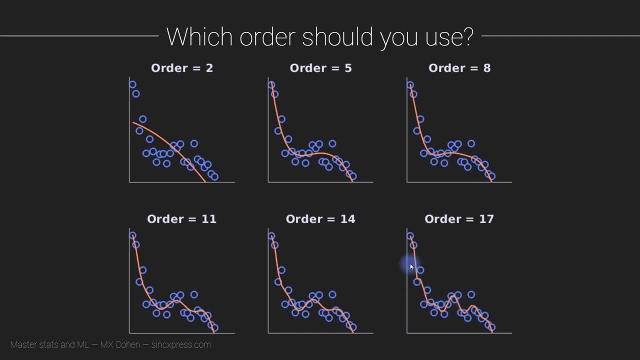 And I showed this slide actually towards the beginning of this course- And this is something about overfitting. We are overfitting data. I'm going to talk more about overfitting in regression modeling soon, in several videos from now. Okay, but so how do we know? 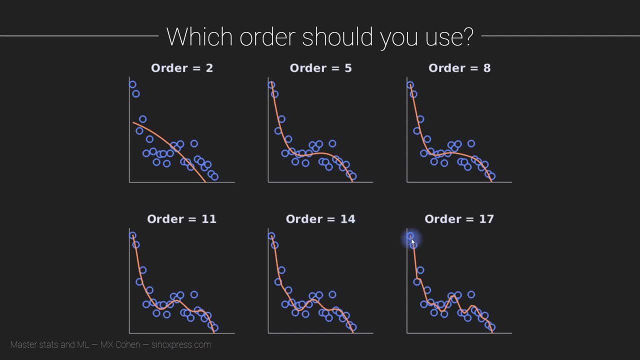 what is the appropriate order that we should use? This is too small. the order is too small Here. the order is too large. We're overfitting. we're capturing too much of noise here. Okay, so the way that we go about figuring out. 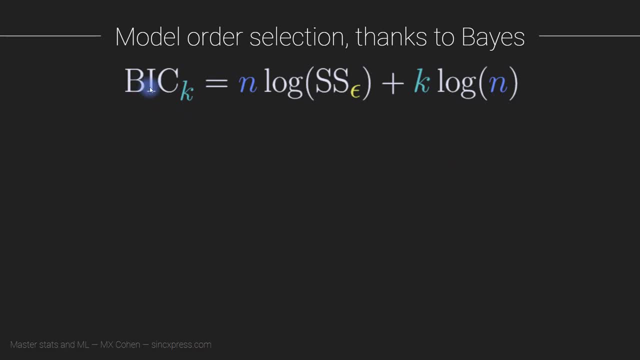 the appropriate order is through something called the Bayes information criteria. It's often just abbreviated as BIC, So this is Bayes information criterion, And so the idea is that this is a quantity that we can compute for every model order. So we get up to K model orders. 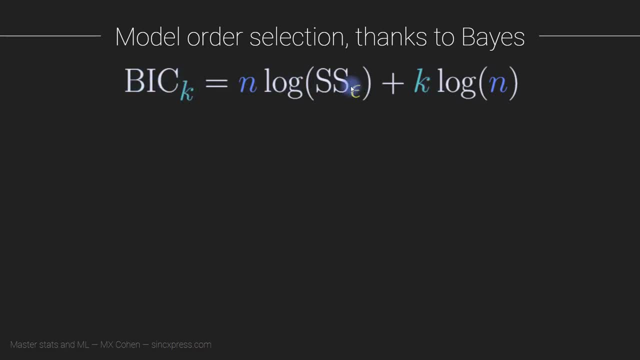 So we can compute K BICs, And this is a formula. So it's N, where N is the number of data points that you have times the log, the natural log of the sum of squares of the residuals, And I showed you the formula for this quantity several times.